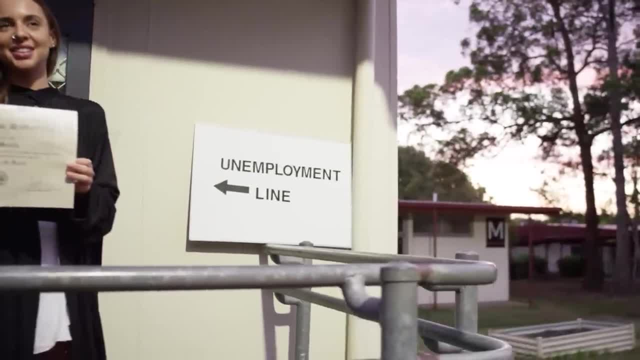 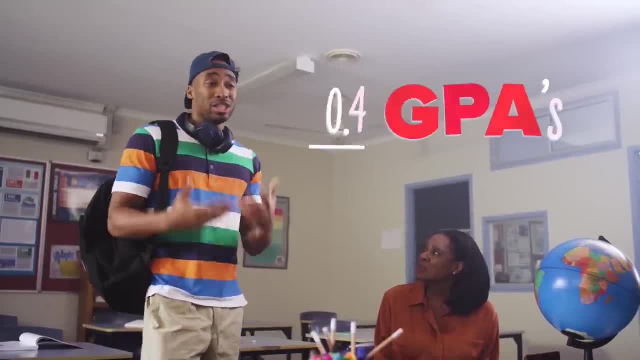 right into the unemployment line. See many top companies today. don't look at grades, Mom. that old way is expiring. Google has been quoted as saying GPAs are worthless criteria for hiring. Founder of Tesla, Elon Musk, agrees. 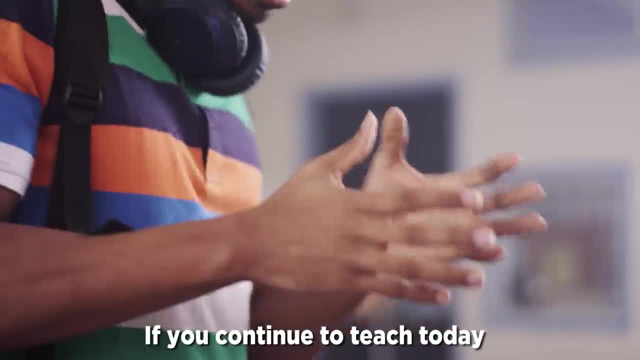 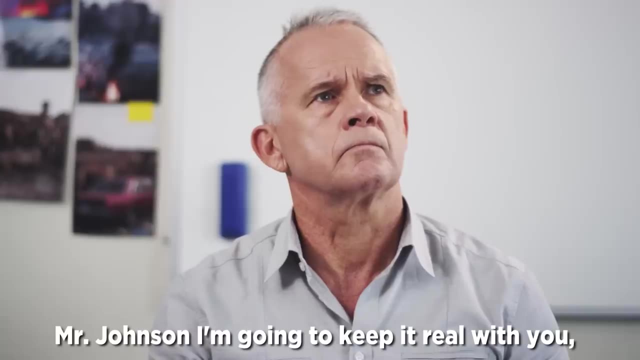 So I say this with unease and sorrow: If you continue to teach today as you taught yesterday, then you rob us students of tomorrow. Mr Johnson, I'm going to keep it real with you. Sometimes sitting in your class is tough. 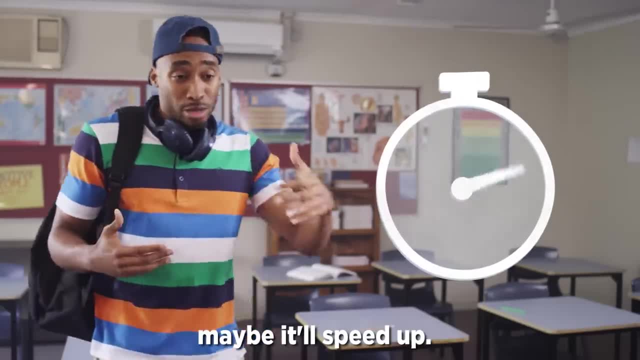 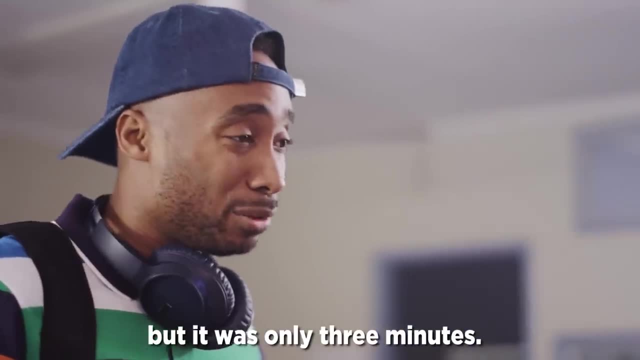 I'm constantly thinking: if I don't look up at the clock, maybe it'll speed up. So I listen to you, Do my homework, Do my work and pay attention, Feeling like an hour had to have gone by, but it was only three minutes. 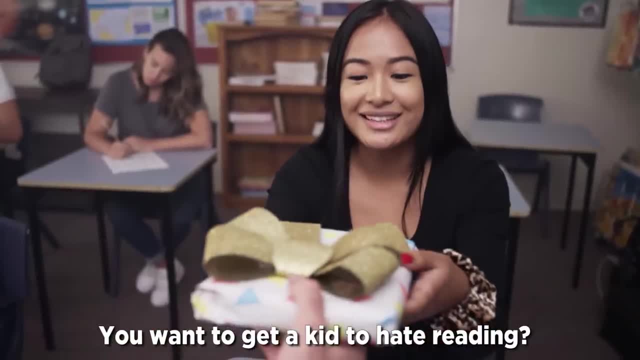 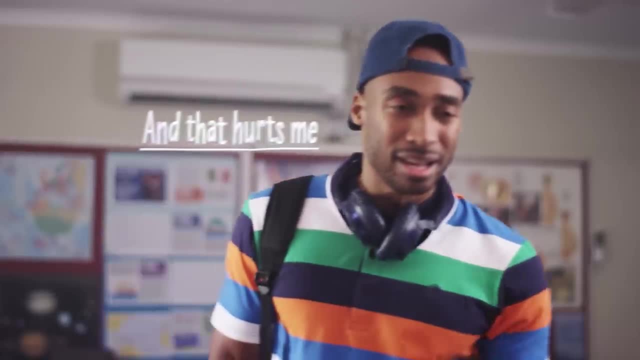 So if you wonder why we're bored in class, look, you want to get a kid to hate reading. Give them this a school textbook. And some people think it's all fault and that hurts me. They say you can lead a horse to water, but you can't make him drink. 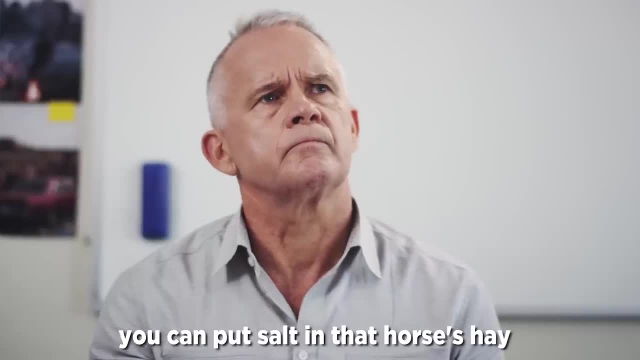 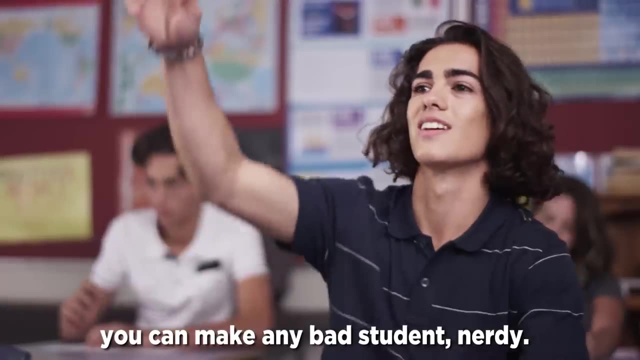 And to that I say no. Firstly, you can put salt in that horse's hay and make him thirsty, And if you bring joy in your classroom, you can make any any bad student nerdy, as he or she discovers the beauty of truly learning. 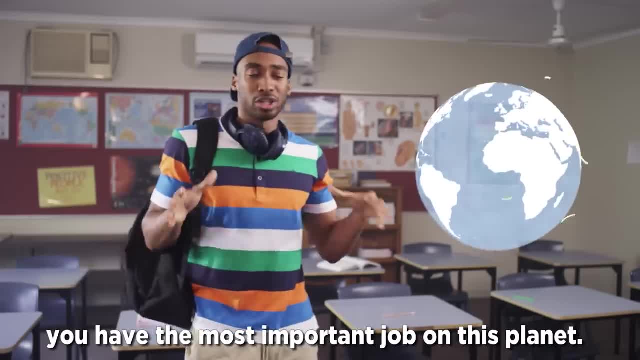 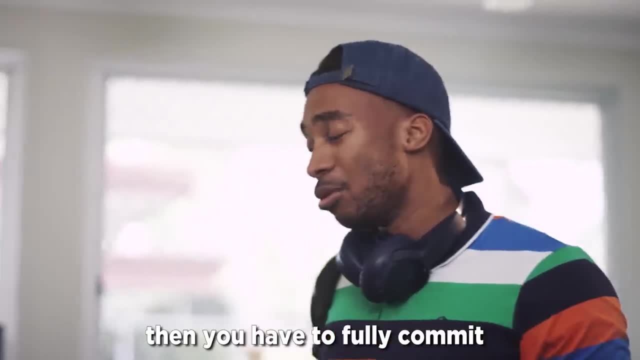 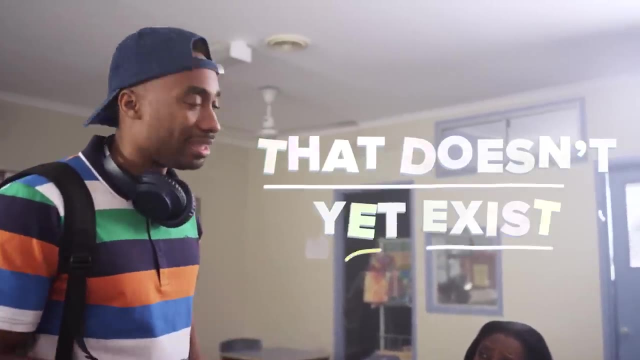 Mr Johnson, I mean no disrespect. You have the most important job on this planet: You build, create and save lives. But if you really care about my future, like you say, then you have to fully commit and ask yourself honestly: how do I prepare a child for a future that doesn't yet exist? 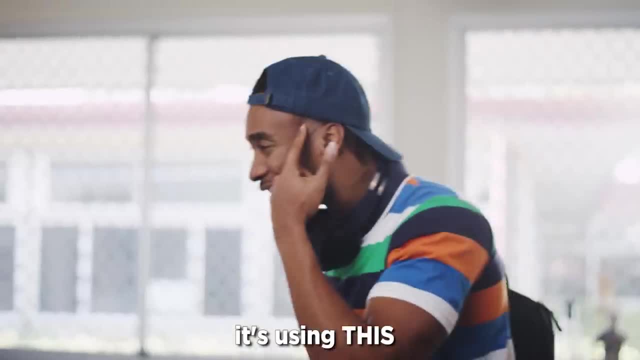 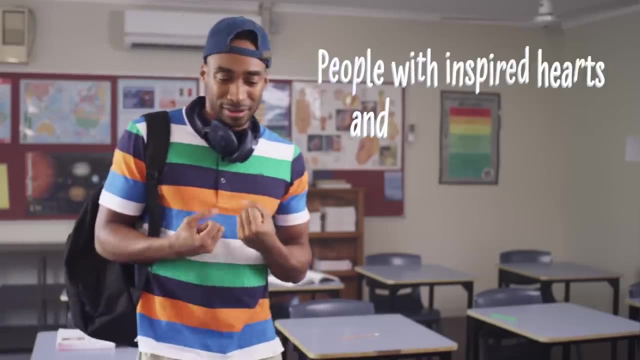 Here's a hint: The answer is not found in this. It's using this and this. See, in the future we will need more passion and compassion, People with inspired hearts and wisdom to uplift this planet. And, mom, I love you, but can I be real? 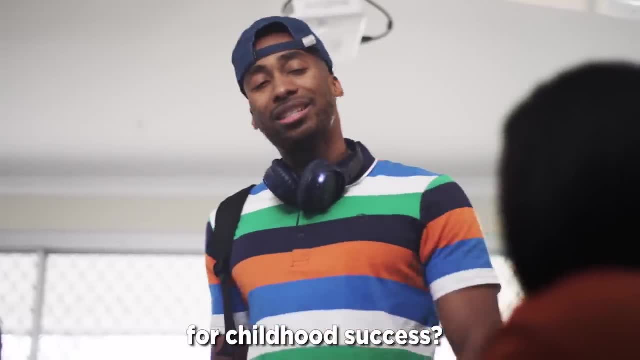 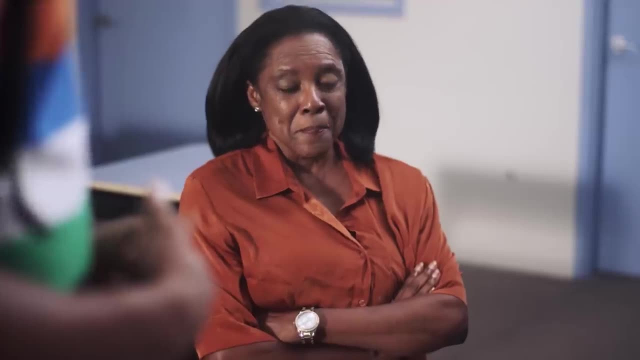 Go ahead. You want to know one of the biggest factors for childhood success. It's not IQ, It's family meals, And we haven't had one of those in a while. See, I know sometimes you don't feel proud because I may not be a straight-A student.